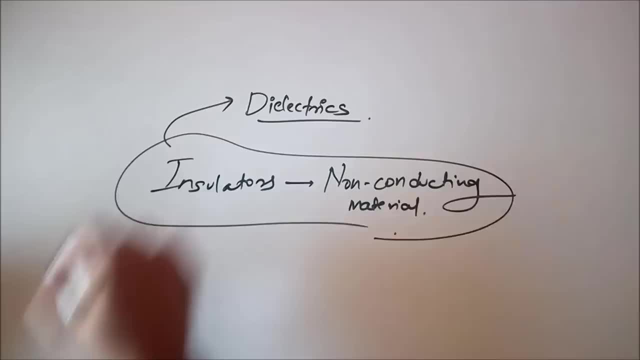 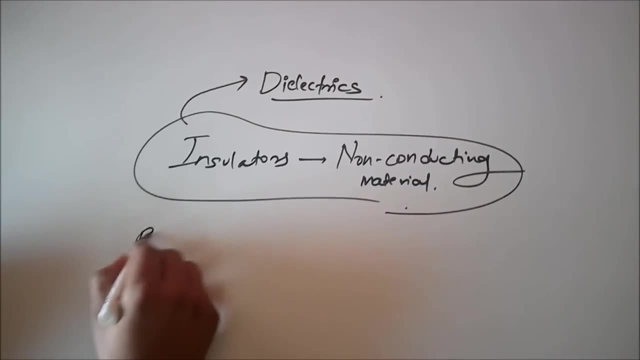 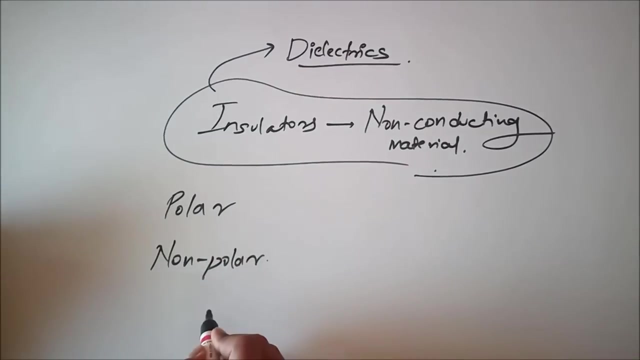 so these materials, whatever are called as dielectrics. dielectrics have two types in mein do type hota hai. the first one is polar aur dusra jo hai. usko, hum log bolte hai non polar, ab mere dielectrics hai do type hai ek hai polar. 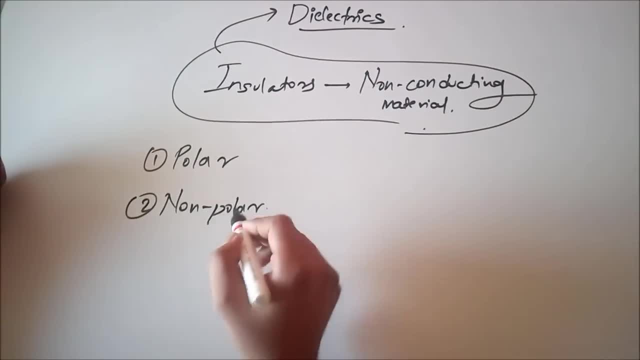 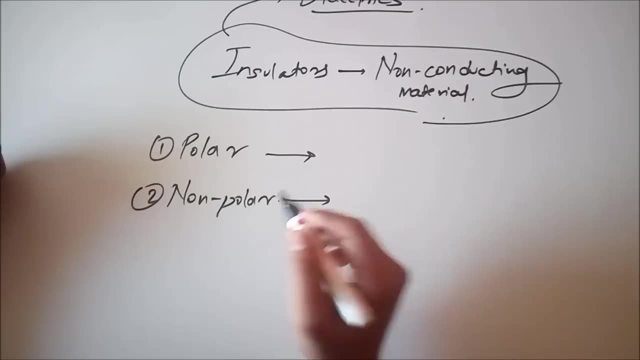 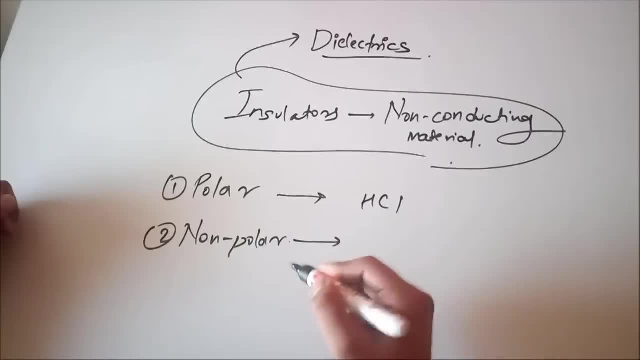 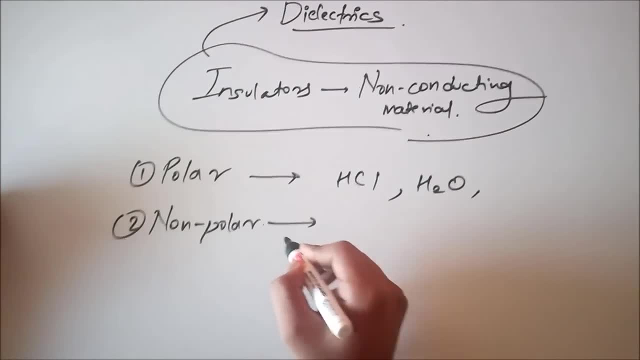 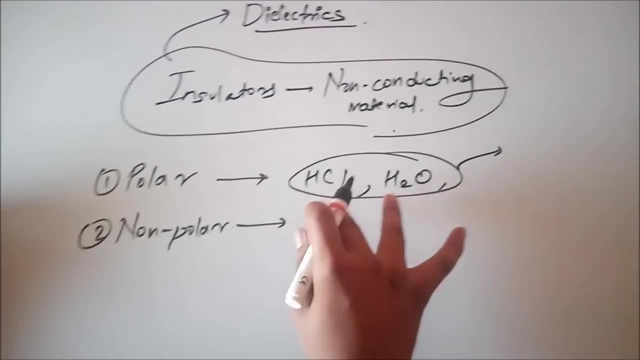 For example, I have HCl. HCL is a polar molecule, then H2O is a polar molecule, and these two molecules are polar molecules. and there are many examples of polar molecules Here. jisa meine bolaki in mein inka dipole: movement jo hota hai, wo constant hota hai. 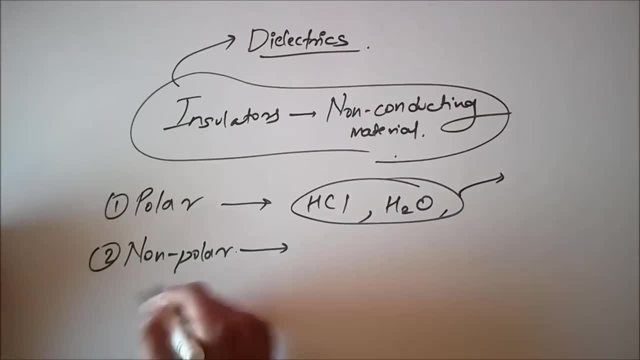 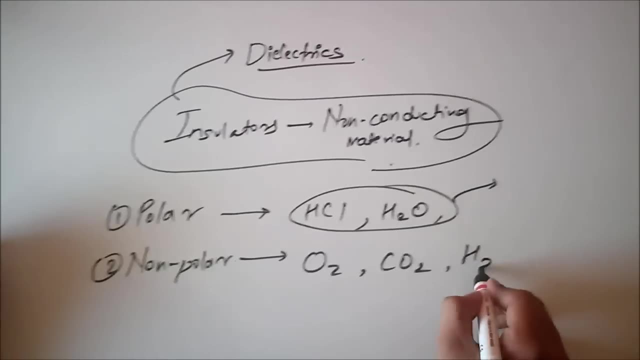 wo change nahi hota, ya pu rok coincide nahi hota. aur non polar ke example. typically, if there is O2, then there is CO2, then H2. these are the frontле and back holes. kye arrival auracement: be j опatka hohe okte ho jops. 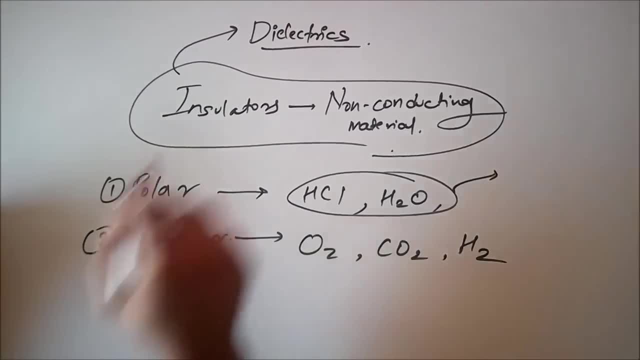 do piero, yo ke es pa advantage nahi mahal ka sameise as this example will break. and What are the examples of non-polar dielectrics? As I said, there are two types of dielectrics: One is polar and the other is non-polar. 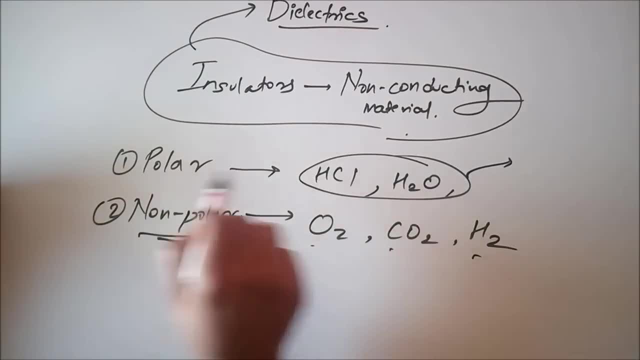 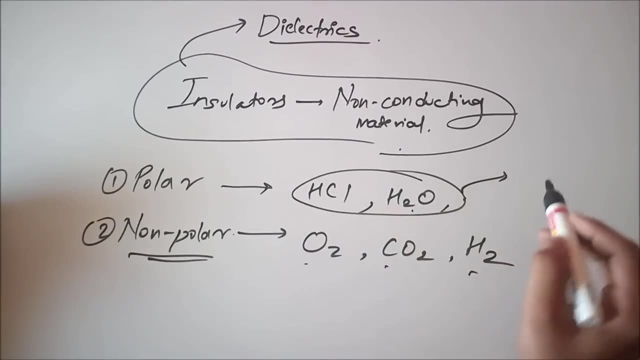 In non-polar I have O2, CO2 and H2.. In polar, I have HCl and O2, H2O. Now I said that their dielectrics, their dipole moment, they don't coincide with each other. 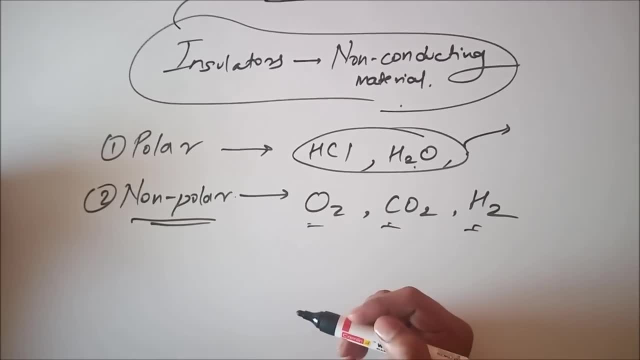 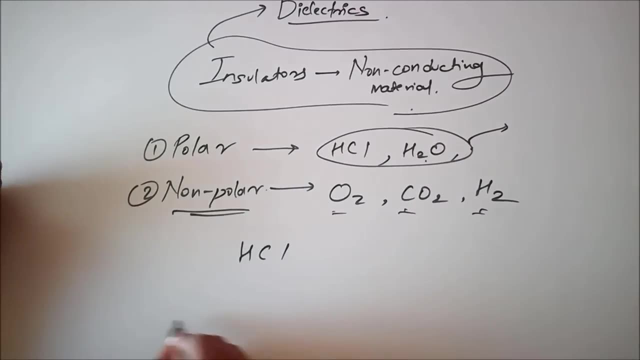 And their dipole moment. they coincide with each other. Now you will have a question in your mind that what is dipole moment? So dipole moment is: suppose I took HCl, Now the molecules of HCl. suppose this is my hydrogen atom and this is my chlorine atom. 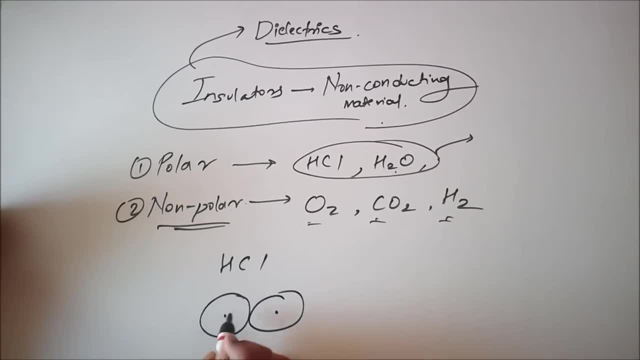 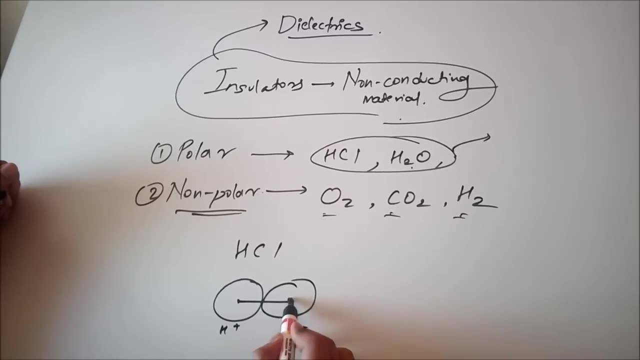 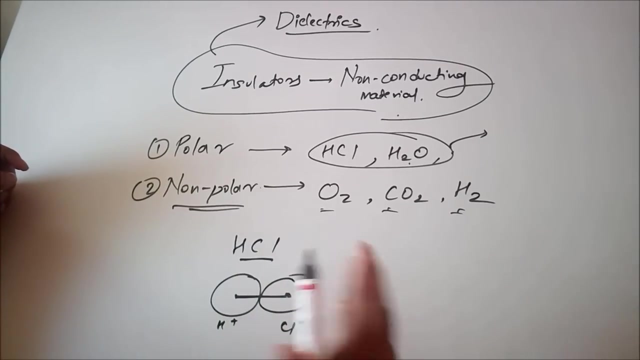 So their central metal atom. from here to here the distance, this is hydrogen and this is chlorine, This is plus and this is minus. So from this center to here the distance we call dipole moment. So here the dipole moment of HCl doesn't coincide with each other. 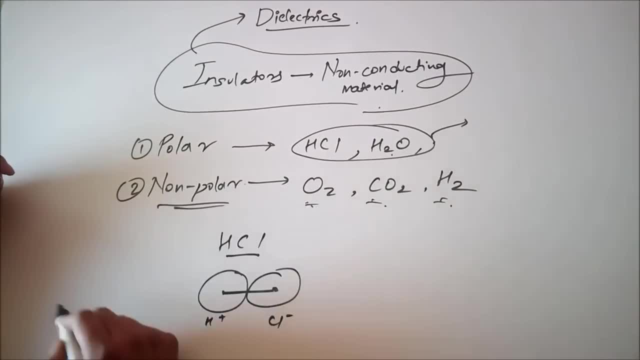 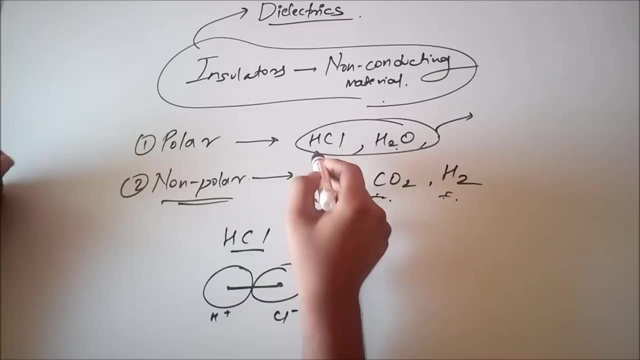 But here, when I talk about non-polar, then here their dipole moment coincides with each other. So there are many different types of materials like this. For example, we took HCl, So these are our liquids. 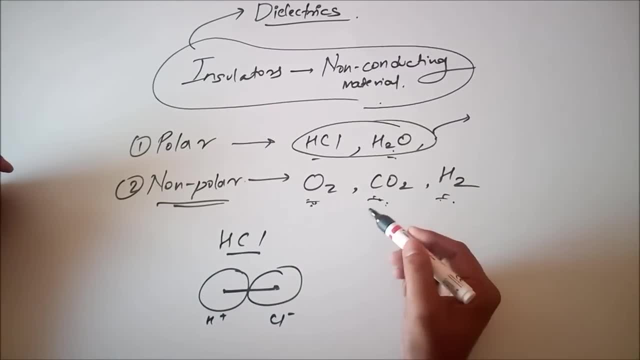 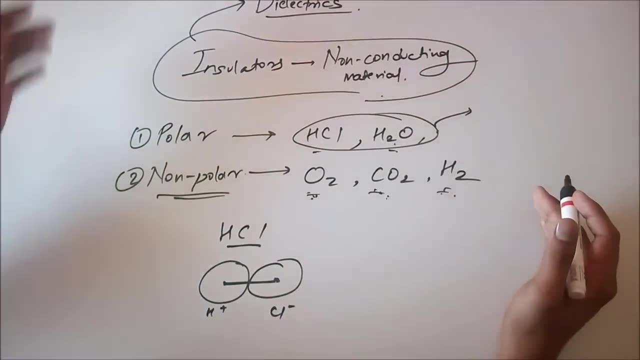 These two are liquids, Then these are our gases. There are many examples like this in solid and liquid gases. Okay, So now these were basically my dielectrics. Now we can use these dielectrics in many types. 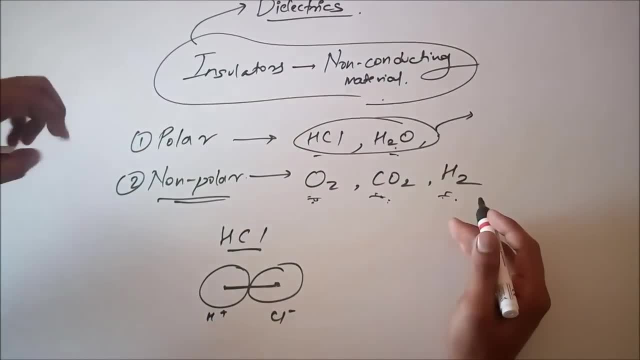 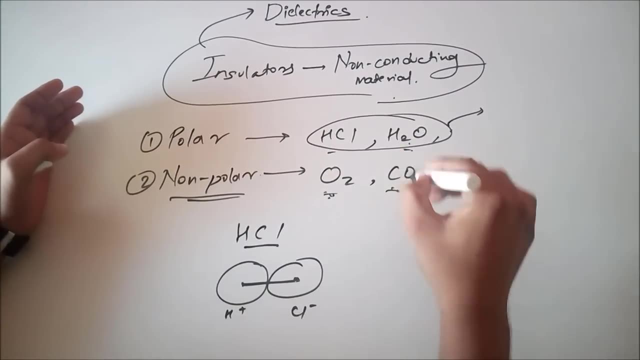 Like when we talk about capacitor. dielectric is used in these dielectrics And how does dielectric work? You will see that in my next video lecture, But today, in these dielectrics, when we place these dielectrics. 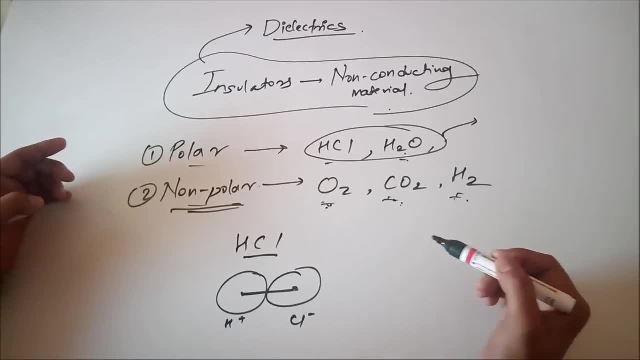 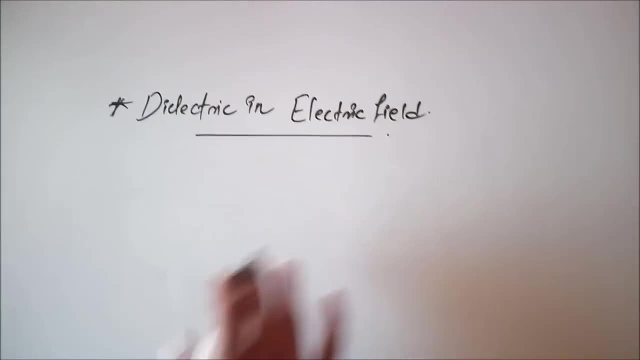 and these dielectrics like polar and non-polar, into an electric field, then what changes do they make? Now, we will see that further. Okay, Now, as we talked about dielectric in electric field, When I keep a dielectric in an electric field, 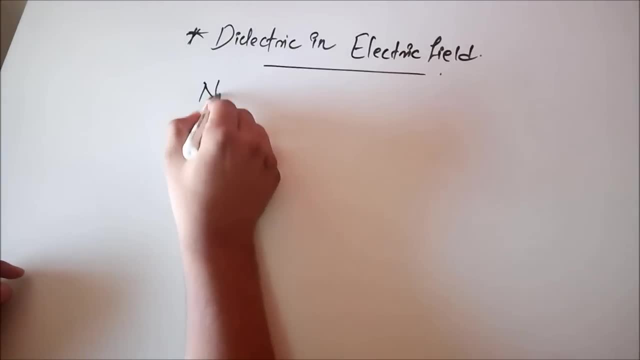 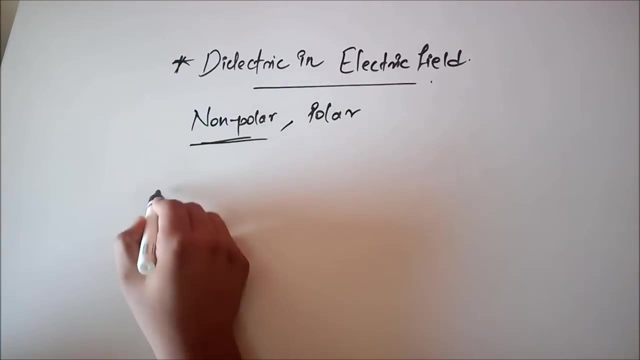 then what changes do they make? Like I told you about my dielectric, I have a dielectric. One is non-polar and the other is polar. So suppose I took any non-polar dielectric field. Suppose I took any non-polar molecule. 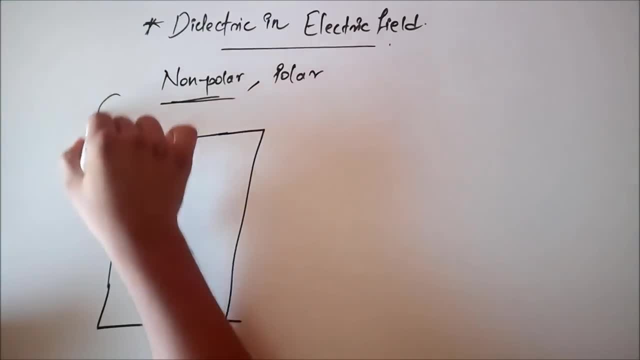 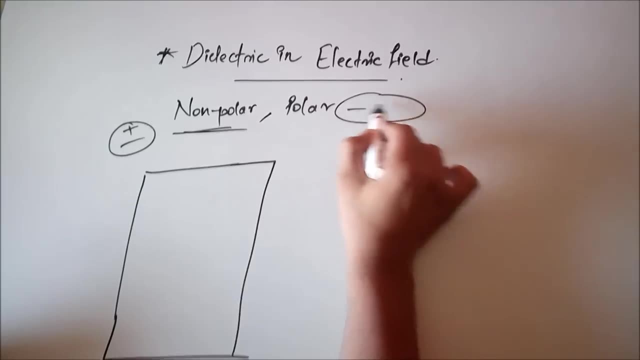 Now I told you that non-polar molecules coincide with each other. That means they will coincide with each other in positive and negative. But what will happen in polar molecules? There will be a dipole moment in between them. That means there will be no coincide between positive and negative. 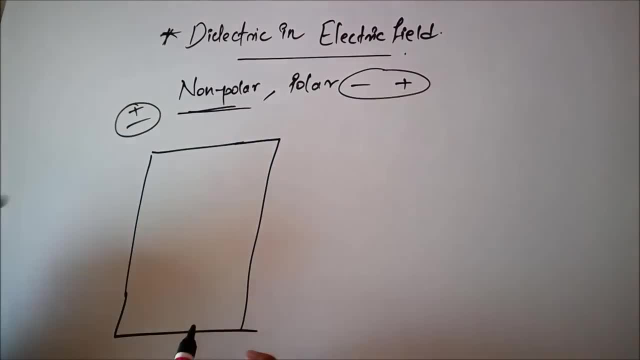 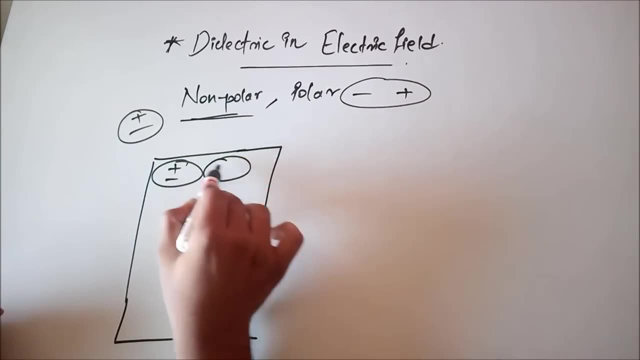 But there will be no dipole moment in between them. So what will they do? They will coincide with each other. Now suppose I have a non-polar molecule. I took a non-polar molecule, Now what are their molecules doing? 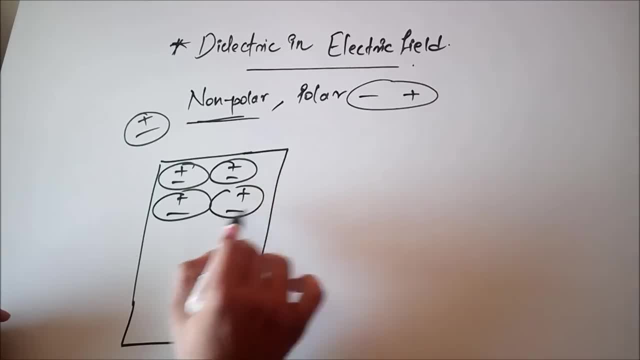 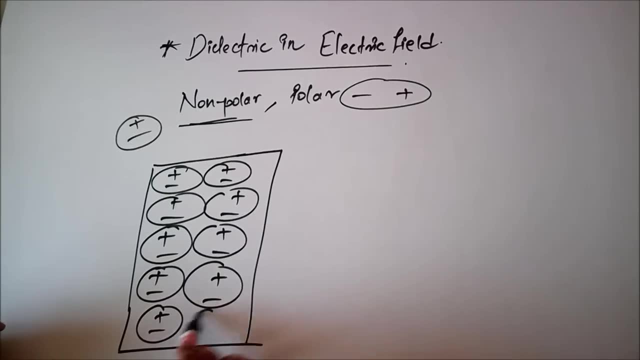 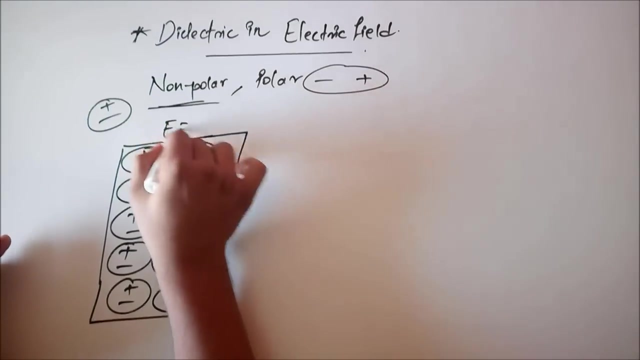 They are coinciding with each other. Suppose I have drawn the molecules. What are they doing? They are coinciding with each other. Okay, I have drawn the molecules, What are they doing? They are coinciding with each other. So if I see here, my electric field is equal to zero. 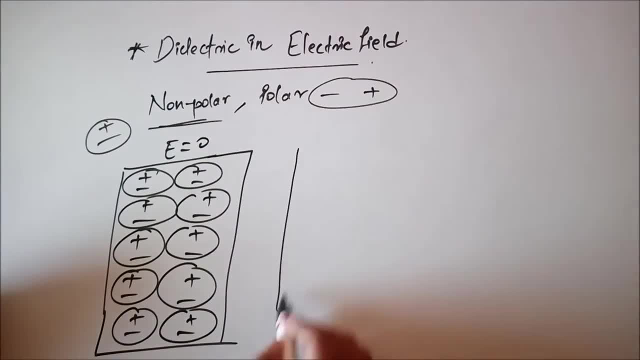 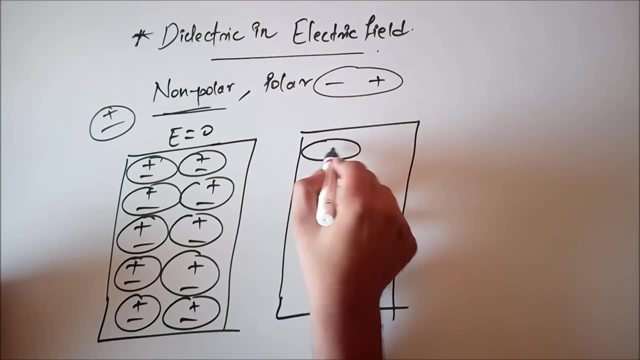 There are no changes in this. But if I take the same molecules, I have taken the same molecules, And when I put the electric field in them there are changes. Here it is positive and here it is negative. That means what happened here. 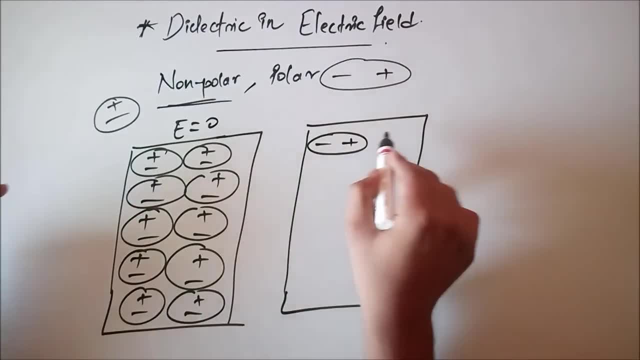 A dipole moment formed in between them. So this is for the first one. So the second one will also be like this: Here it is negative and here it is positive. It will be like this: below Negative, positive. 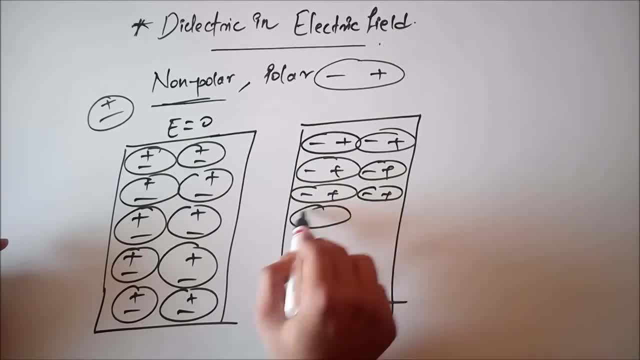 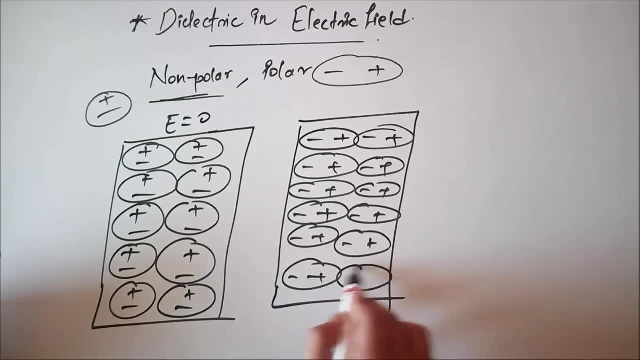 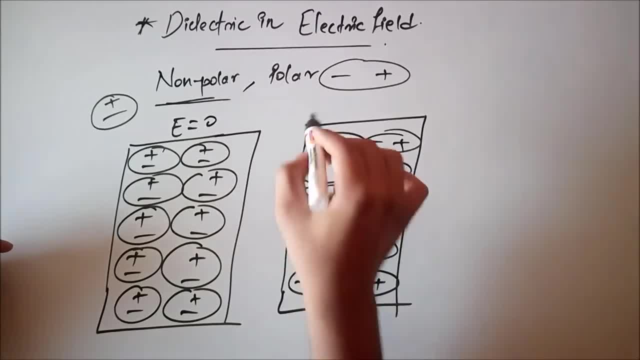 Earlier there was no dipole moment. But now what happened here? A dipole moment formed. So what did I do here Here? I sent an electric field, Suppose. originally I sent an electric field, I named it Evo. 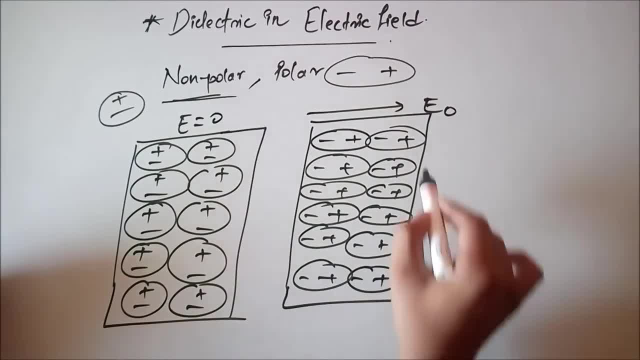 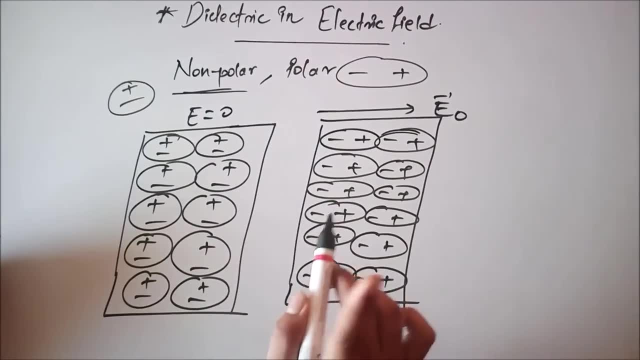 So in this way I sent many electric fields here. So I sent my electric field. But now what happened here? Here, the dipole moment formed. Because of them. what happens Here? another electric field is generated. 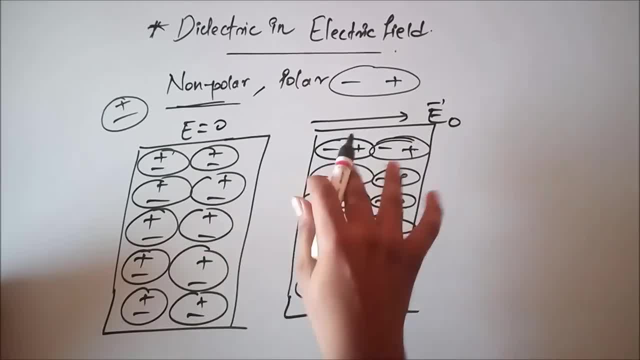 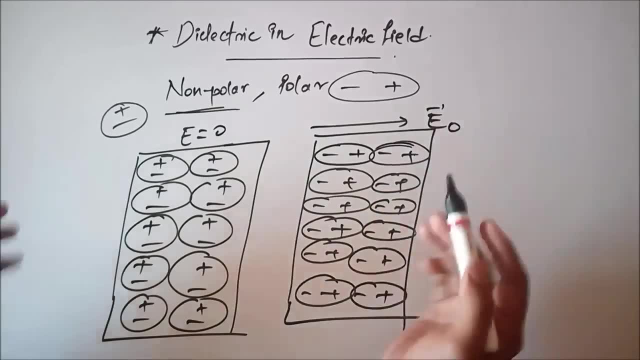 And this electric field is generated due to the dipole moment Of this non-polar molecule. Now, this dipole moment formed here. What will happen from here? Electric field will be generated And we know electric lines flow from positive to negative. 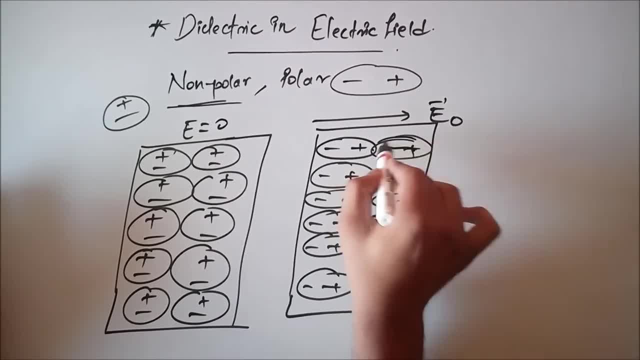 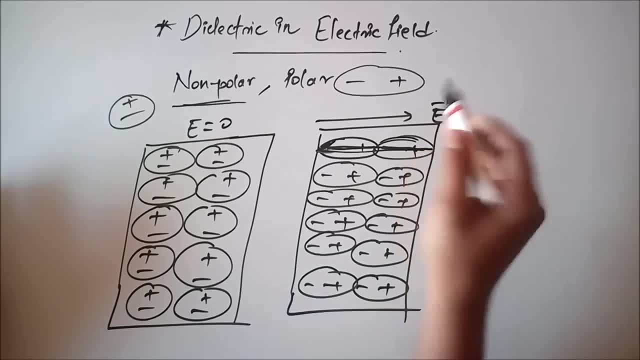 So where will my electric lines of charge go? Positive to negative, Again, positive to negative, That means what? From here, an electric field is generated, And how is it going? From right to left? It is going from right to left. 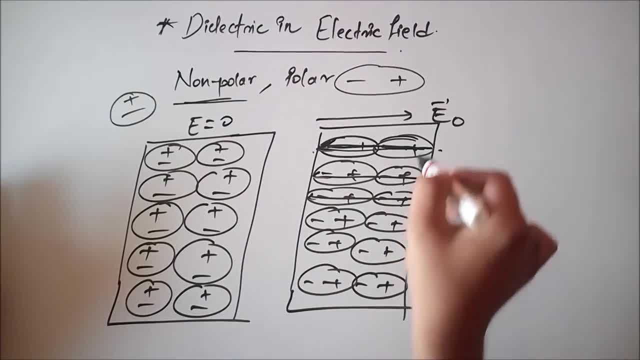 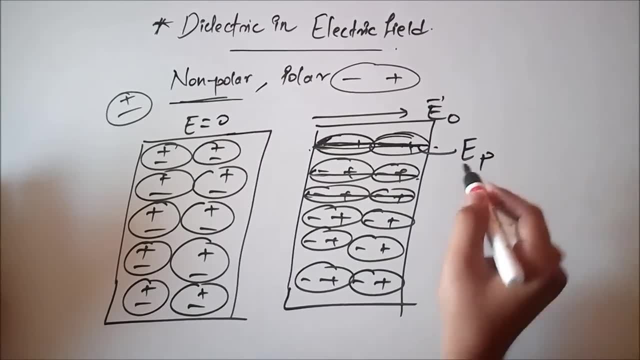 So similarly, this will also happen. Similarly, this will also happen. That means here another electric field is generated, And this electric field is generated due to polarization. For this, the electric field generated here, we will name it EP. 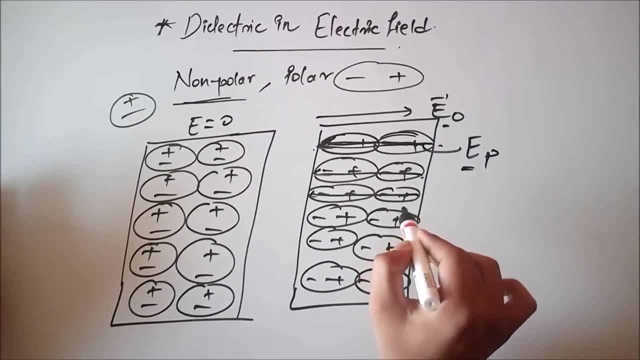 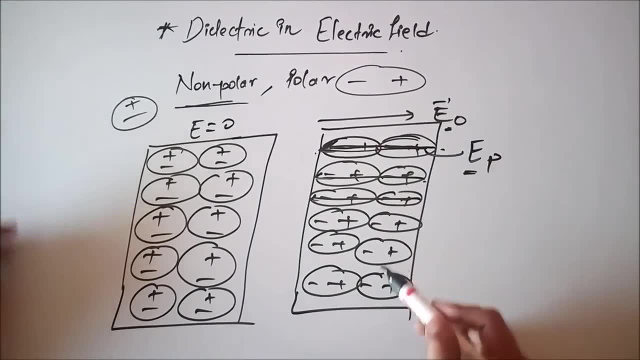 And this was my original electric field. Okay, So here again my electric field is generated, And this electric field is opposite in direction with respect to my original electric field. So here my total electric field, or E net electric field. what will happen?